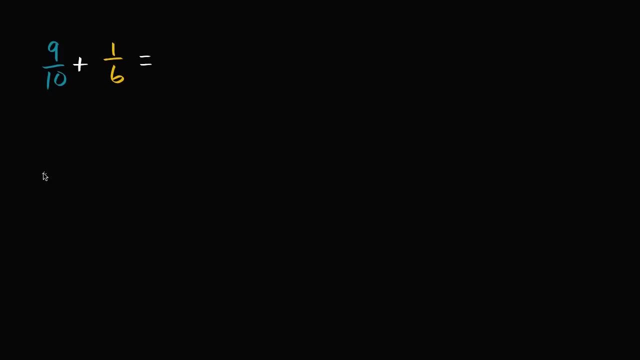 So I can rewrite both of these fractions as something over 30.. So nine over 10, how would I write that as something over 30?? Well, I multiplied the denominator. I'm multiplying the denominator by three. So I've just multiplied the denominator by three. 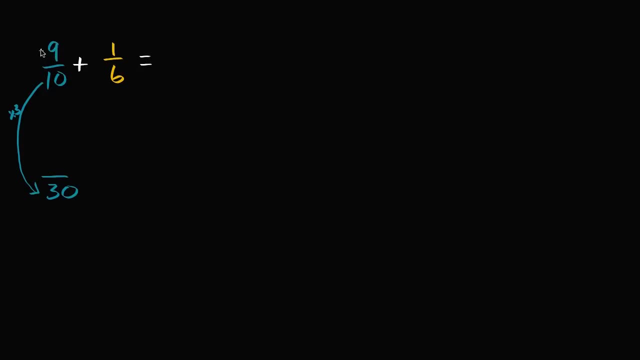 So if I don't wanna change the value of the fraction, I have to do the same thing to the numerator. I have to multiply that by three as well, because now I'm just multiplying the numerator by three and the denominator by three, and that doesn't change the value of the fraction. 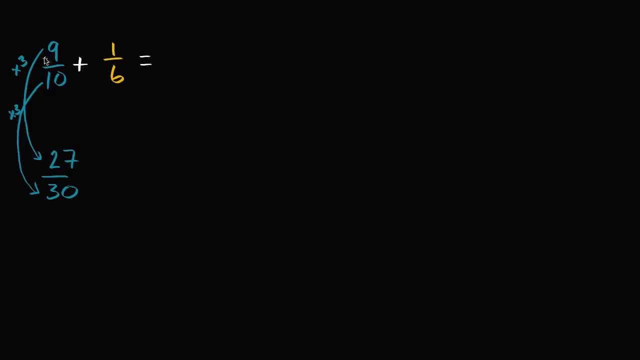 So nine times three is 27.. So once again, nine-tenths and 27-thirtieths represent the same number. I've just written it now with the denominator of 30, and that's useful because I can also write. 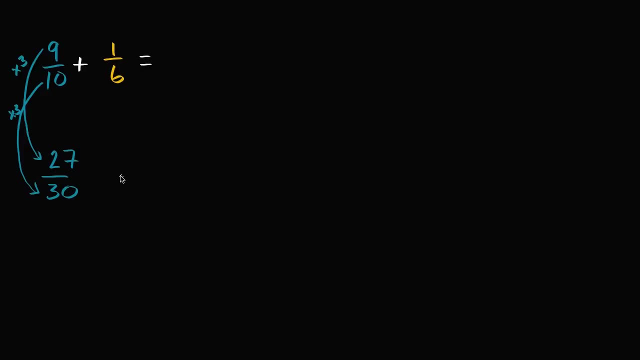 one-sixth with the denominator of 30. Let's do that. So one-sixth is what? over 30?? And I encourage you to pause the video and try to think about it. So what did we do to go from six to 30?? 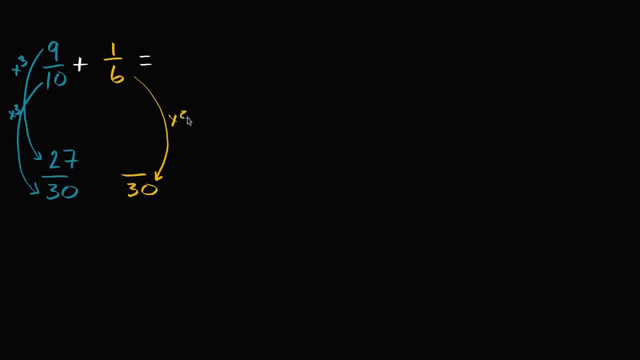 We had to multiply by five. So if we multiply the denominator by five, we have to multiply the numerator by five as well. So one times five is five. So nine-tenths is the same thing as 27-thirtieths. 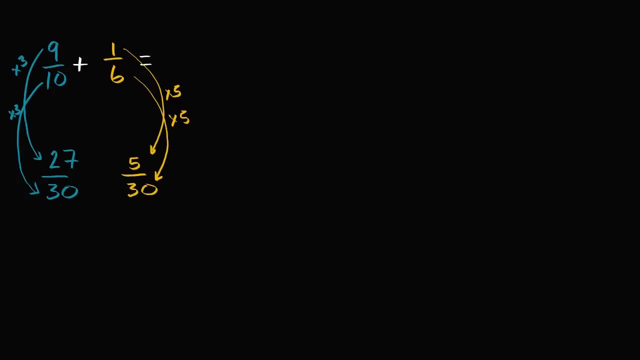 and one-sixth is the same thing as five-thirtieths, And now we can add. Now we can add, and it's fairly straightforward: We have a certain number of 30-ths added to another number of 30-ths. 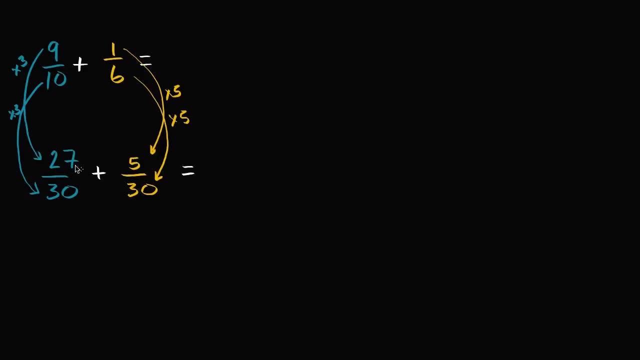 So 27-thirtieths plus five-thirtieths, well, that's going to be 27 plus five-thirtieths, which, of course, is going to be equal to what is this? 32-thirtieths? 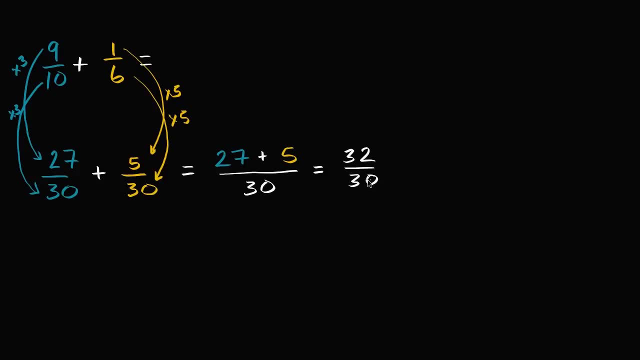 32 over 30. And if we want, we could try to reduce this fraction. We have a common factor of 32 and 30. They're both divisible by. let's see, they're both divisible by two. So if we divide the numerator and the denominator by two, 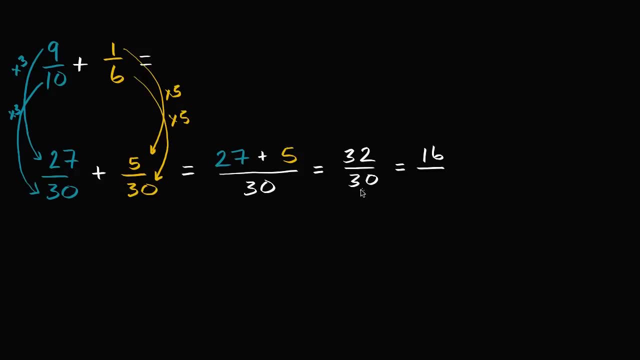 numerator divided by two is 16.. Denominator divided by two is 15.. So this is the same thing as 16-fifteenths, And if I wanted to write this as a mixed number, 15 goes into 16, one time with the remainder one. 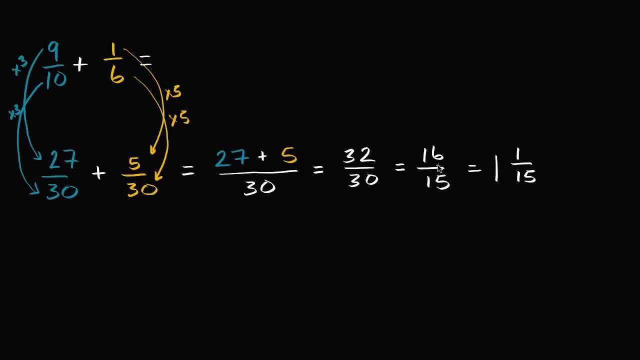 So this is the same thing as one and one-fifteenths. Let's do another example. Let's say that we wanted to add, we wanted to add one-half, one-half, two to 11-twelfths, To 11 over 12.. 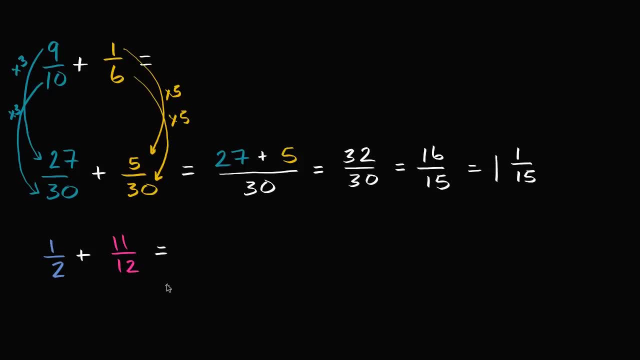 And I encourage you to pause the video and see if you can work this out. Well, like we saw before, we want to find a common denominator. If these had the same denominator, we could just add them immediately, But we want to find a common denominator. 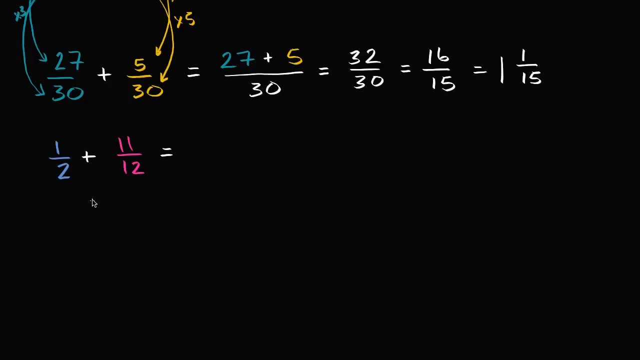 because right now they're not the same. Well, what we want to find is a multiple, a common multiple of two and 12.. And ideally, we'll find the lowest common multiple of two and 12.. And, just like we did before, let's start with the larger of the two numbers: 12.. 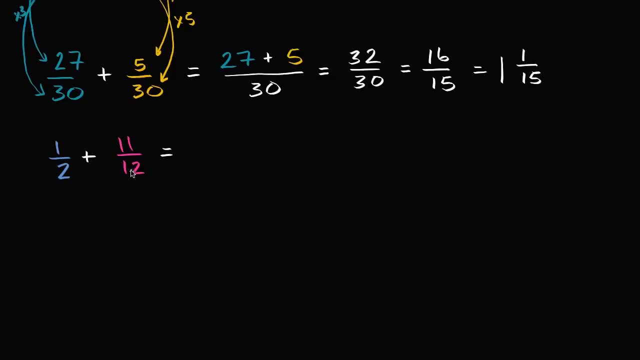 And we could just say: well, 12 times one is 12, so you could view that as the lowest multiple of 12.. And is that divisible by two? Yeah, sure, 12 is divisible by two. So 12 is actually the least common multiple of two and 12.. 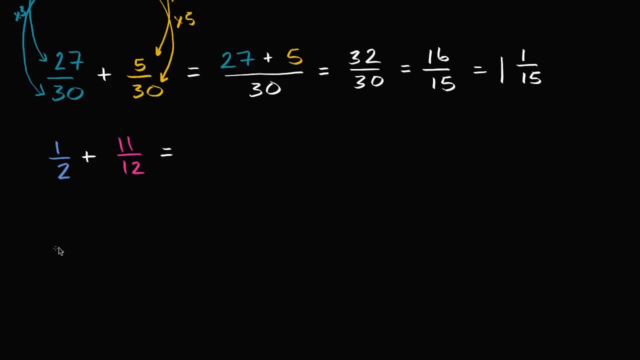 So we could write both of these fractions as something over 12.. So one-half is what over 12?? Well, to go from two to 12, you multiply by six. So we'll also multiply the numerator by six And we see one-half and six-twelfths. 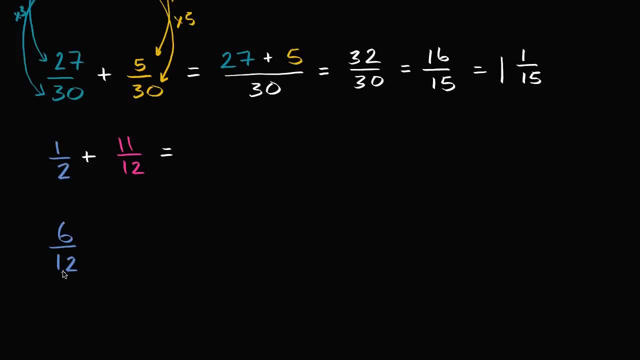 these are the same thing. One is half of two, six is half of 12.. And how would we write 11-twelfths as something over 12?? Well, it's already written as something over 12.. 11-twelfths already has 12 in the denominator. 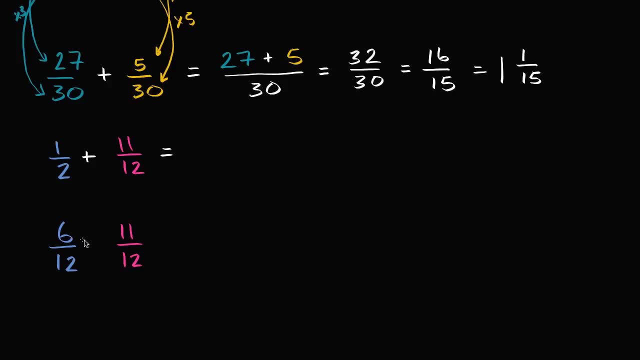 so we don't have to change that. 11-twelfths, and now we're ready to add, So this is going to be equal to six. This is going to be equal to six plus 11.. Six plus 11 over 12, over 12.. 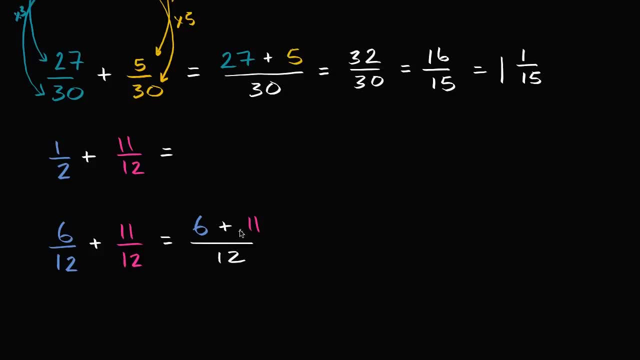 We have six-twelfths plus 11-twelfths is going to be six plus 11 over 12.. Which is equal to six plus 11 is 17-twelfths, If we want to write it as a mixed number. 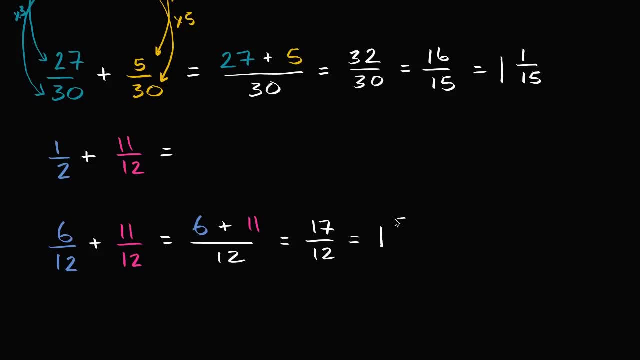 that is what 12 goes into: 17 one time with the remainder five. So one and five over 12.. Let's do one more of these. This is strangely fun. Alright, let's say that we wanted to add. we're going to add three-fourths to. 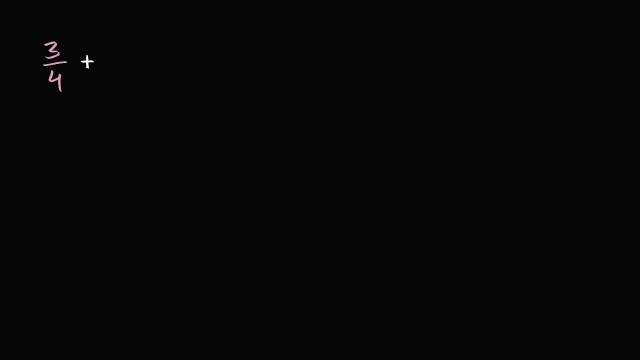 we're going to add three-fourths to one-fifth, To one over five. What is this going to be? And once again, pause the video and see if you can work it out. Well, we have different denominators here and we want to find, we want to rewrite these.